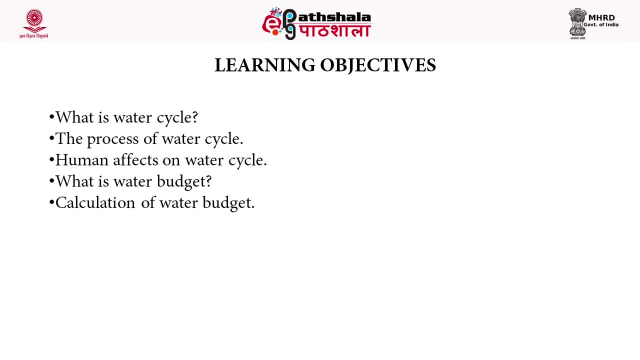 cycle. what are the various factor which affect the water cycle? Moreover, we will also discuss about water budget. What is water budget? How can we calculate water budget of any area And what are the various factor which affect the water budget? Now we discuss in detail. 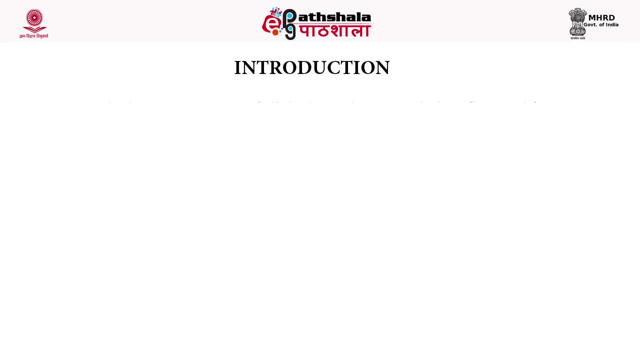 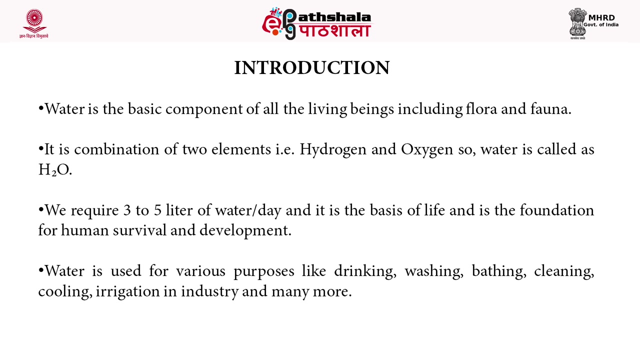 Introduction: water is the basic component of all the living being, including flora and fauna. It is combination of two elements, that is, hydrogen and oxygen, So water is called as H2O. We require three to five liter of water per day, And it is the basis of life and is the foundation for human survival and development. Water. 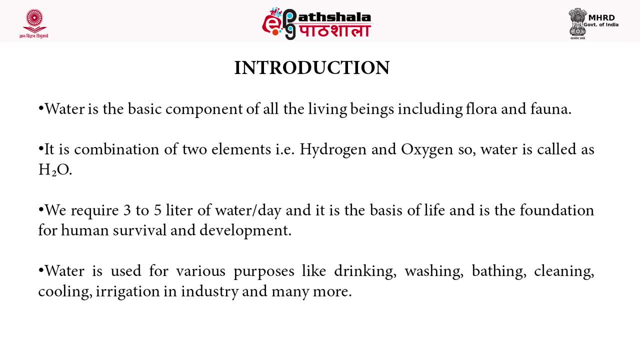 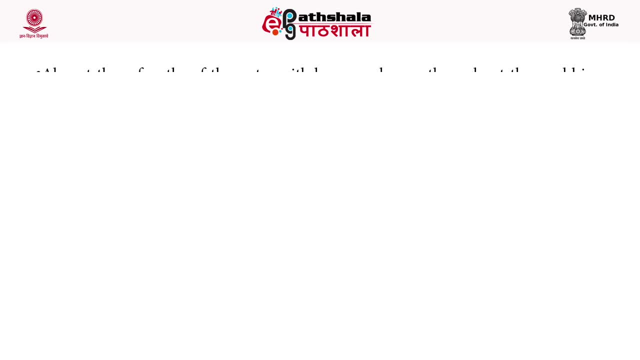 is used for various purposes, like drinking, washing, bathing, cleaning, cooling, irrigation in industry and many more. Almost three-fourths of the water withdrawn each year throughout the world is used for irrigation. The remainder is used for industrial processing, energy production, cooling, electric power plants, for domestic and industrial activities About. 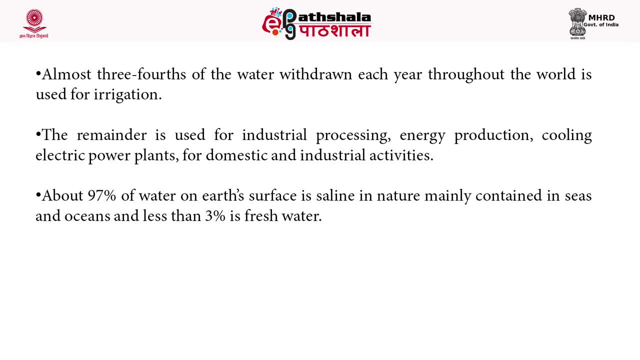 ninety-seven percent of water on earth. earth surface is saline in nature, mainly contained in seas and ocean, and less than three percent is fresh water. The sources of fresh water on earth include the precipitation, surface water, that is, stream, rivers, sandstone, which. 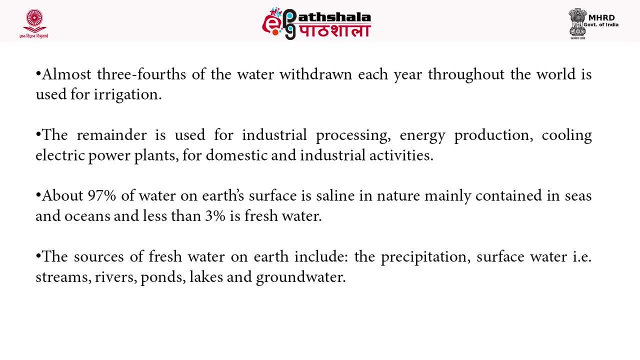 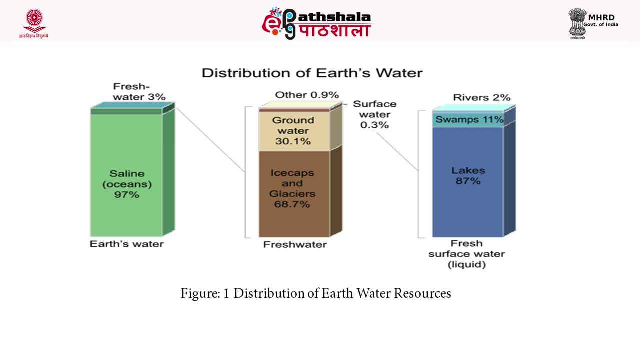 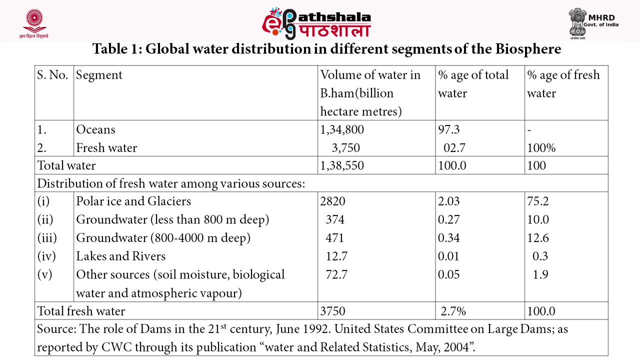 is turned into of biogas, flora, fauna and fauna. The position of groundwater is in two pond lakes and ground water. The figure 1 shows the distribution of earth water resources on earth. From table 1, we can see that ocean consists of maximum water on earth surface. 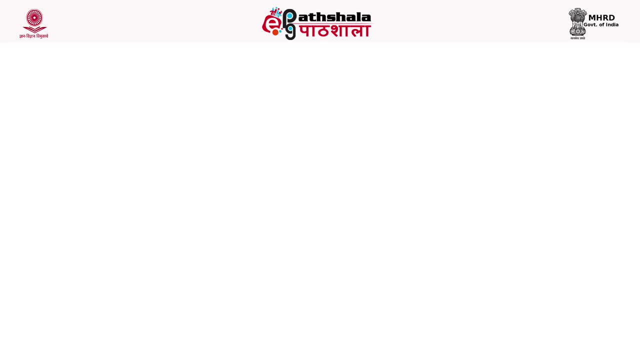 and fresh water is limited. About 97.3% water is saline in nature and contained in ocean. It cannot be used for domestic purpose, ie for drinking, washing, cooking and bathing, etc. Moreover, fresh water is also used for irrigation, for industrial activity and energy. 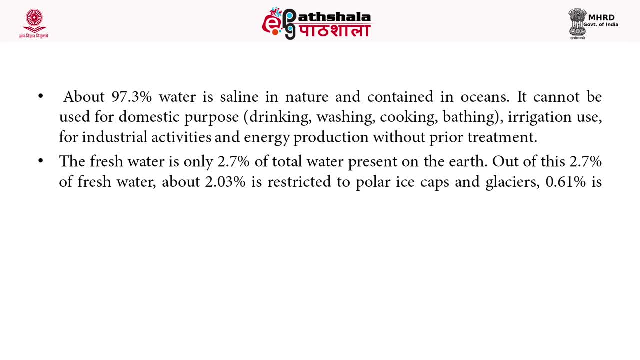 production. The fresh water is only 2.7% of total water present on earth. Out of this 2.7% of fresh water, About 2.03% is restricted to polar ice caps and glacier. 0.61% is present underground. 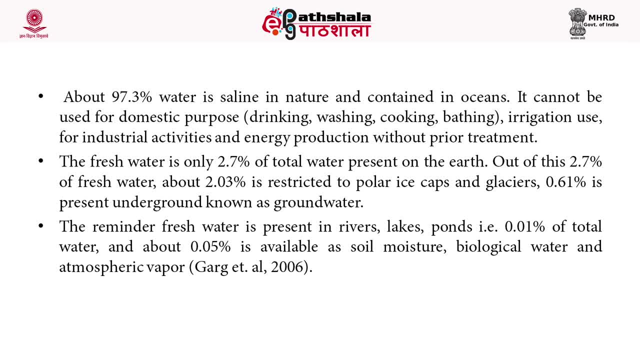 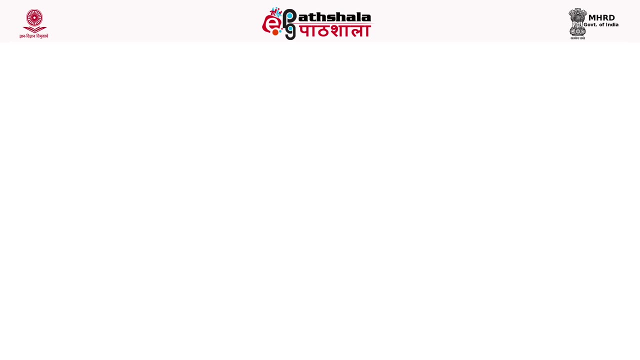 known as ground water. A reminder: fresh water is present in rivers and lakes and ponds, ie 0.1% of total water, and about 0.05% is available as soil, moisture, biological water and atmospheric vapor. Now we will discuss about water cycle, ie hydrological cycle. 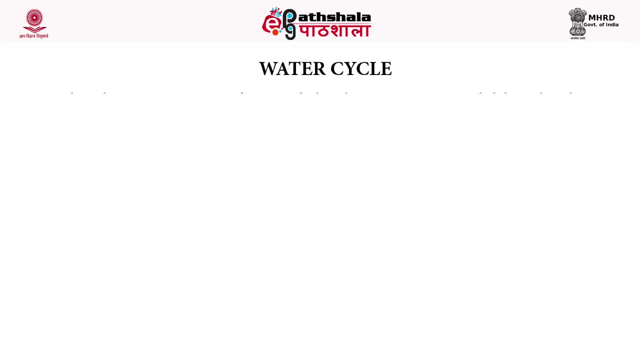 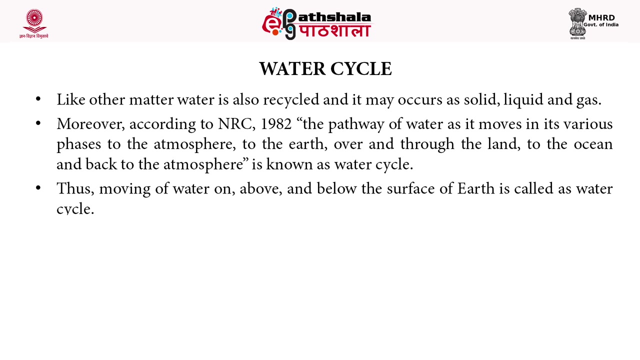 In water cycle, the water comes in a regular form, matter. water is also recycled and it may occur as solid, liquid and gas. ie water exists in all three states of matter. Moreover, according to the National Research Council, water cycle may be defined as the pathway of water as it moves in its various phases. 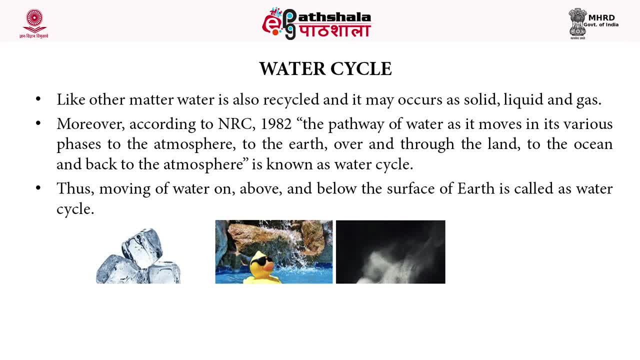 to the atmosphere, to earth, over and through the land, to the ocean and back to atmosphere, is known as Water Cycle, or in other word we can say cycling of water from earth's surface to atmosphere, from atmosphere to earth's surface. this cycling of water is known as. 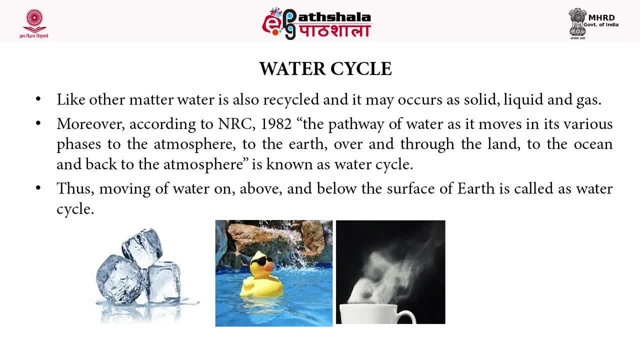 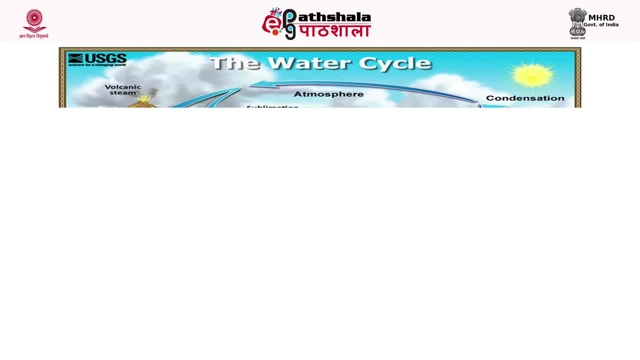 Water Cycle, Thus moving of water on above and below the surface of earth to earth, has been described as a cycle of water. Thus, what are the Muslim earth is called as water cycle. Figure 2 show the diagram of water cycle, how water enter. 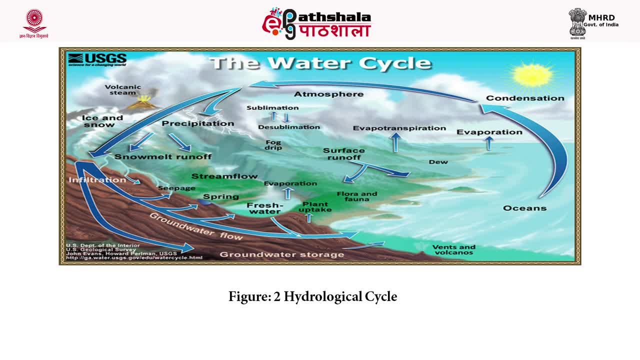 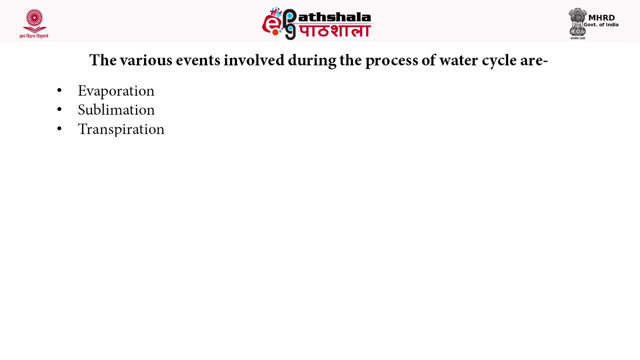 to atmosphere, how from atmosphere it come back to earth. various event occur in the process of water cycle are shown in figure 2.. The various events which occur in water cycle are evaporation, sublimation, transpiration, precipitation, infiltration, percolation. 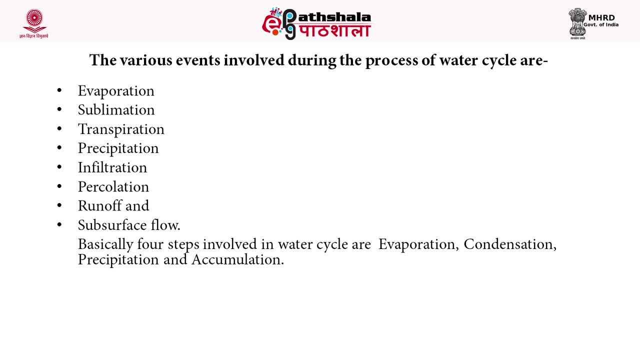 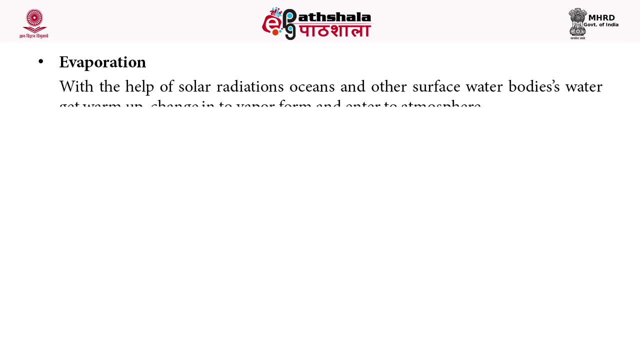 runoff and subsurface flow. Basically, four steps involved in water cycle are evaporation, condensation, precipitation and accumulation. Now we will discuss one by one these major event. Number one: evaporation With the help of solar radiation, ocean and other surface water. 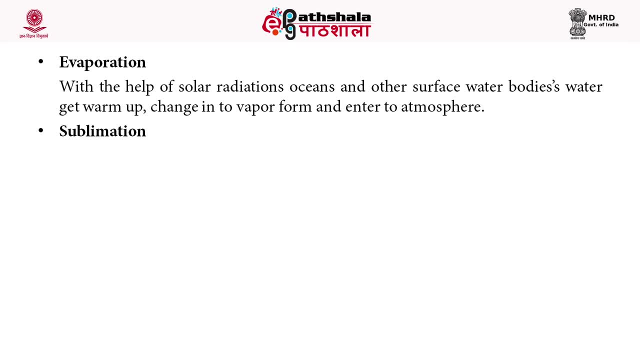 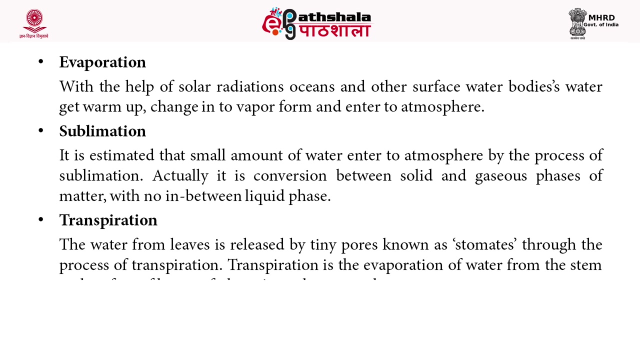 body bodies. water get, warm up, change into vapor form and enter to atmosphere. This process is known as evaporation. That is, sun is the main power which provides water to water cycle. Number two, sublimation. It is estimated that small amount of water enter to atmosphere by the process of sublimation. 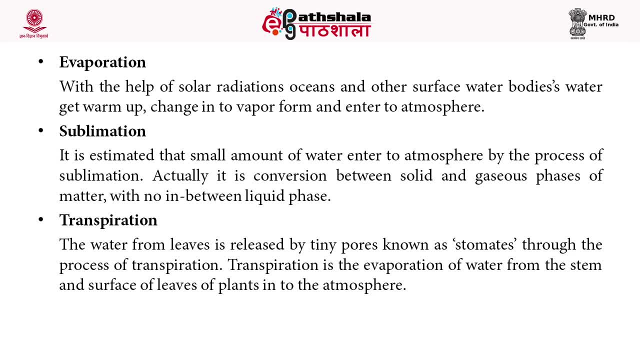 Actually it is conversion between solid and gaseous phase of matter, with no in between liquid phase, That is directly. water in vapor form enter to atmosphere through ice, etcetera. Transpiration: The water is Water from leaves or plants is released by tiny pores known as stomatae, through the process. 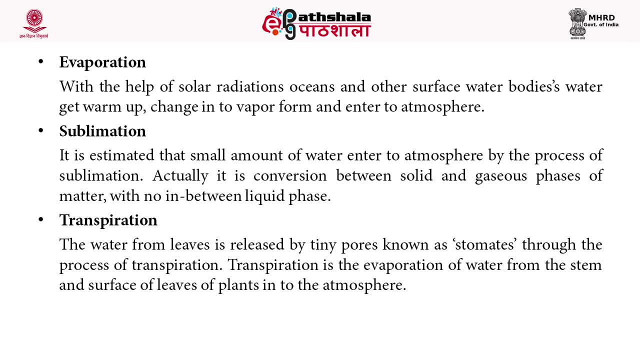 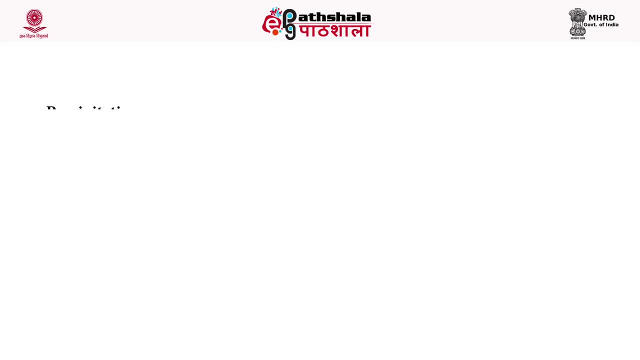 of transpiration. Transpiration is the evaporation of water from the stem and surface of leaves or plants in the atmosphere. Precipitation- It is the main source of fresh water supply to the entire world, and it may occur in liquid or solid form. The water vapors get condensed and, under the influence of gravity, these 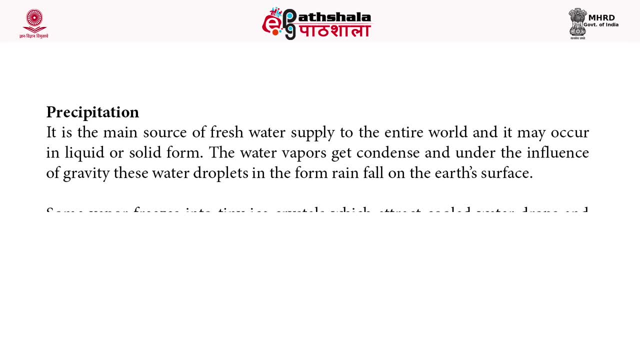 water droplets in the form of rain fall on the earth's surface, ie falling of rain or, in solid form, hail, etc. Some vapor freezes into tiny ice-cream crystals which attract cooled water droplets. Water drops and may fall as hail or snowfall, known as freezing rain. Thus, most of the 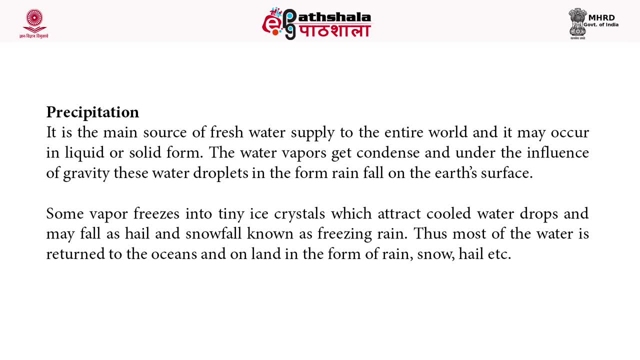 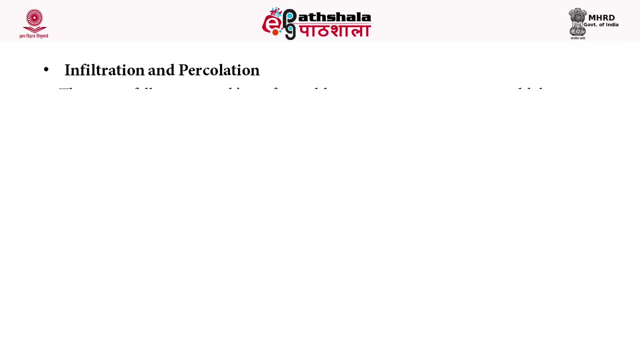 water is returned to the ocean and on land in the form of rain, snow, hail, etc. Infiltration and percolation The water falling on earth's surface add water to rivers, streams and lakes, etc. The water from these water bodies and land seeps to ground. 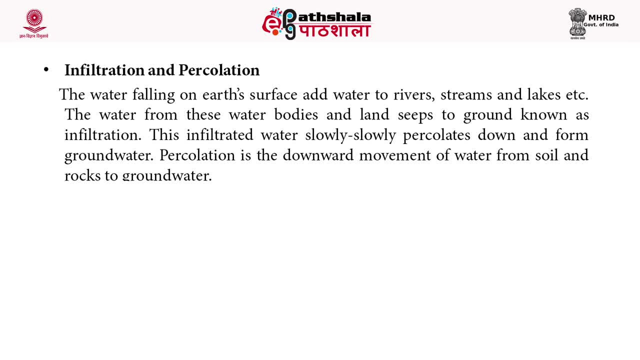 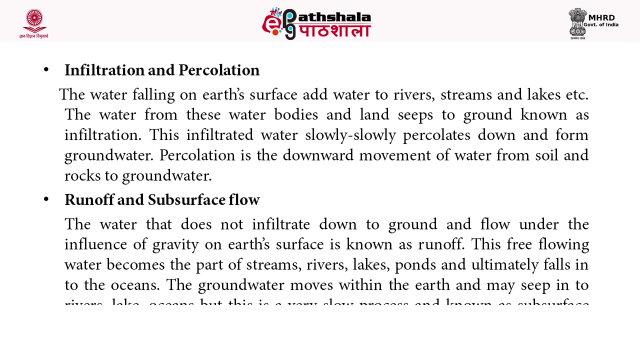 known as infiltration. This infiltrated water slowly, slowly percolates down from ground water. Percolation is the downward movement of water from soil and rocks to ground water, Runoff and subsurface flow, The water that does not infiltrate down to ground and flow. 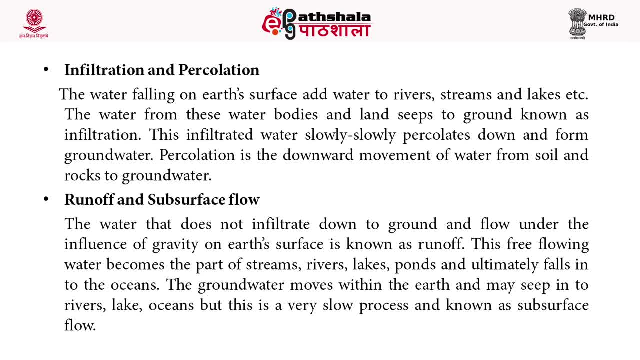 under the influence of gravity on earth's surface is known as runoff. This furry flowing water becomes the part of stream, river, lakes, ponds and ultimately falls into the ocean. The ground water moves within the earth and may seep into river, lake, ocean. but this 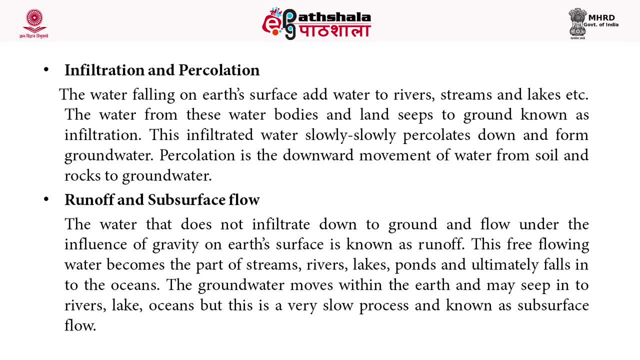 is a very slow process and known as subsurface flow, That is, water moves within the earth and may seep into river, lake, ocean. but this is a very slow process and known as subsurface flow, That is, water moves within the earth. 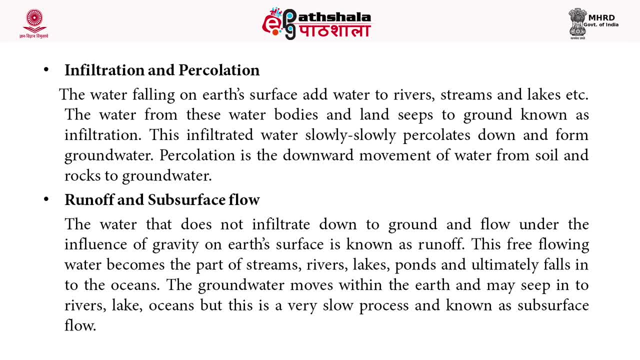 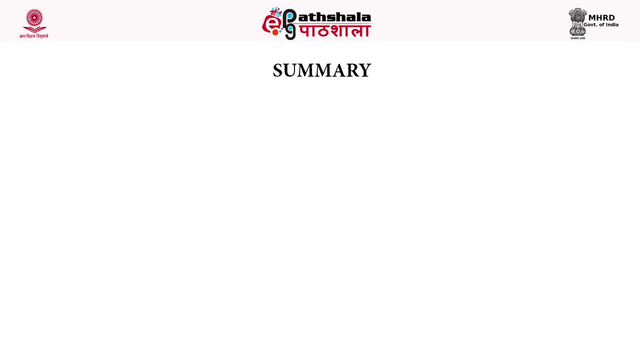 moving below the surface of earth is known as subsurface flow. Now, summary of water cycle. The major source of water on earth are rainfall, surface water and ground water. However, water cycle, that is, hydrological cycle, recycles the earth's precious fresh water supply. that is the main source of fresh water supply on earth: Water. 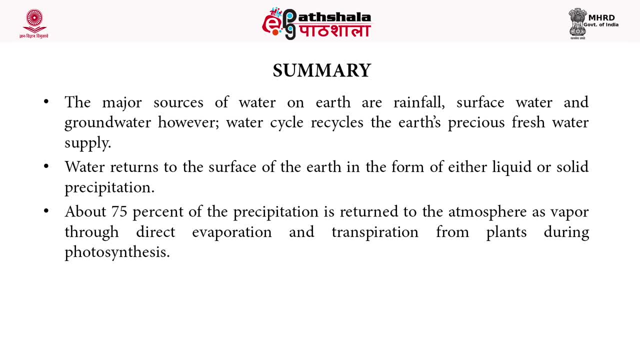 return to the surface of earth in the form of either liquid or solid precipitation, that is, hail, ice, snow, etcetera. About 75 percent of the precipitation is returned to the atmosphere as vapor through direct evaporation and transpiration from plants during photosynthesis. 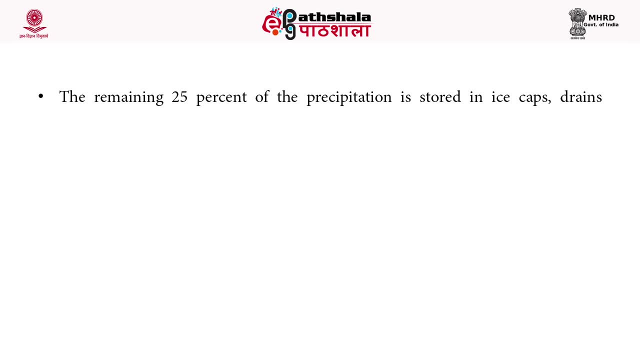 Now the remaining 25 percent of the precipitation is stored in ice caps. drains directly. it drains directly of the land into the lakes, streams, wetland, river and ocean, or infiltrate the soil and underlying rock layers and enter the ground water system That is remaining. 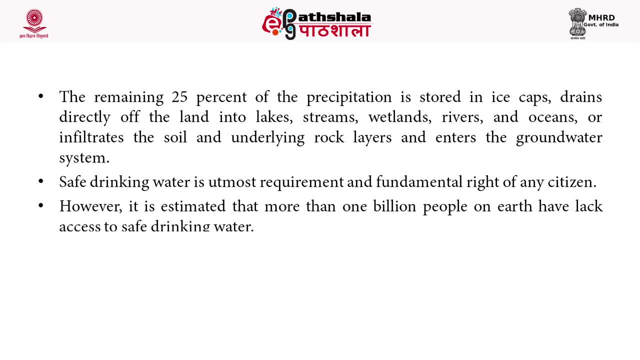 water slowly, slowly infiltrate into the soil and provide water to ground water. Safe drinking water is utmost requirement and fundamental right of any citizen. However, it is estimated that more than 1 billion people on earth have lack access to safe drinking water. Human activities affecting the water cycle, for example. 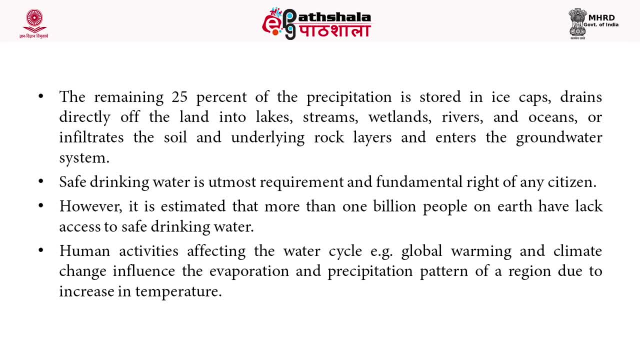 global warming and climate change influence the evaporation and precipitation pattern of region due to increase in eutrophication of water In recent years. the warmest of the earth's population is an average of 6.6 percent, but its average global warming Along. 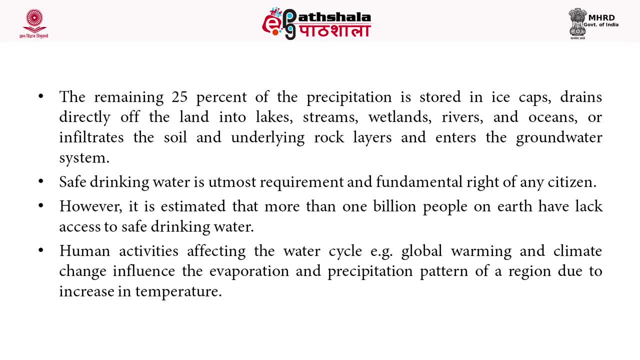 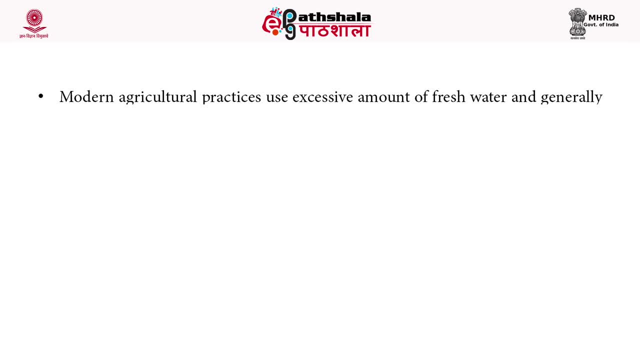 the horizon is the highest in the continent size. The most abundant source of water is temperature. Moreover, deforestation also affects the water cycle. Modern agricultural practices use excessive amounts of fresh water and generally rely on groundwater That is the most precious resource for fresh water on earth. The excessive withdrawal of groundwater. 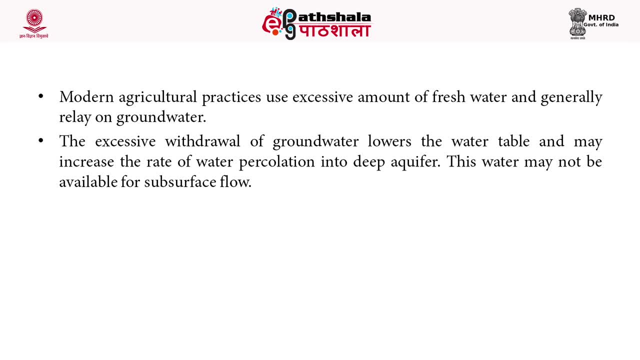 lowers the water table and may increase the rate of water percolation into deep aquifer. This water may not be available for subsurface flow. Aquifers are the regions from where we can extract groundwater, Layer of sand, sediment, etc. which hold the water is known. 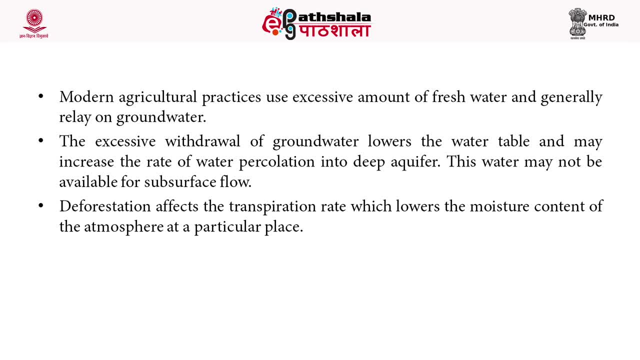 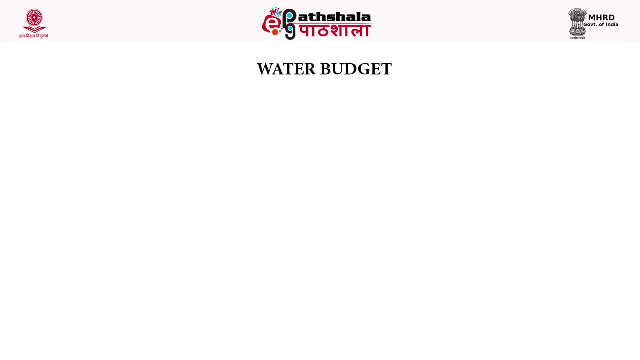 as aquifer. Moreover, deforestation also affects the transpiration rate, which lowers the moisture content of water. Now we will discuss about water budget. What is the meaning of water budget? The balance between available water and the water under use of a specific region, that is, it is balance. 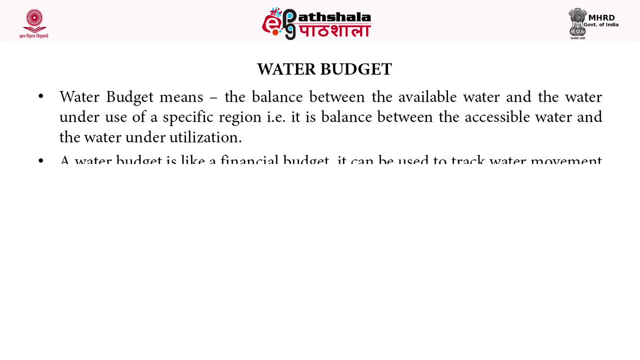 between the accessible water- accessible means easily available- and water under utilization. Moreover, a water budget is like a financial budget. It can be used to track water movement through the water cycle. Here, precipitation is the income and evaporation transpiration. 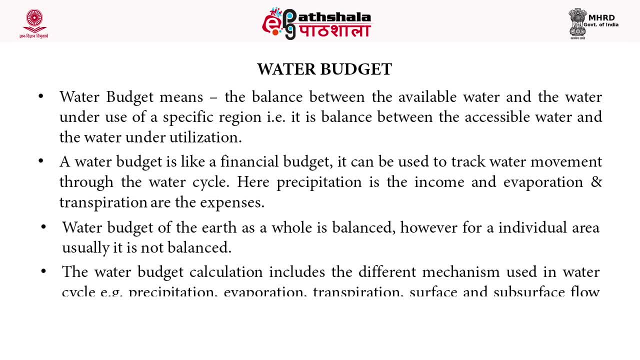 are the expenses. Water budget of the earth as a whole is balanced. However, for a individual area usually it is not balanced due to various natural conditions. Water budget can also influence the unbalancing of land frozen served by the standardIn certain areas. water costs. 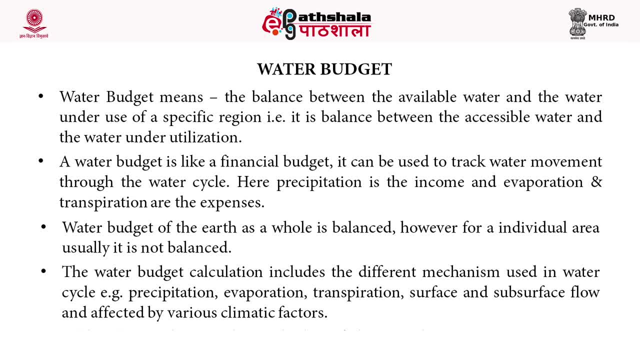 are another consideration, ie while naturally water costs are not important, However, water budget may be itself to be considered as purelyelen required. water budget for arrangement is only natural as well as human activity. The water budget calculation includes the different mechanism used in water cycle, that is, precipitation, evaporation, transpiration, surface and subsurface. 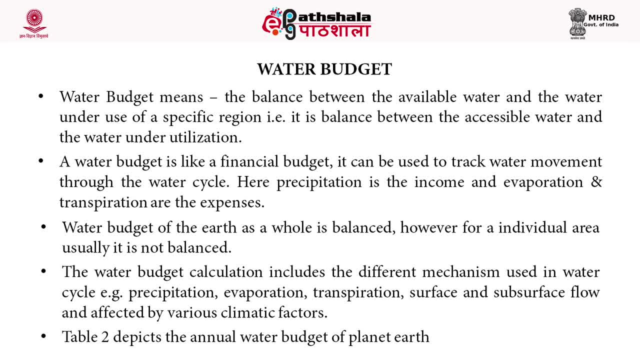 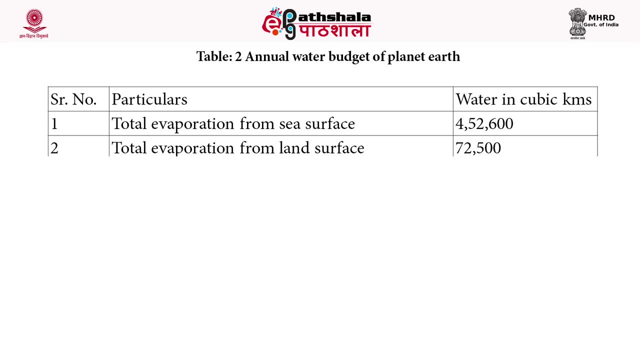 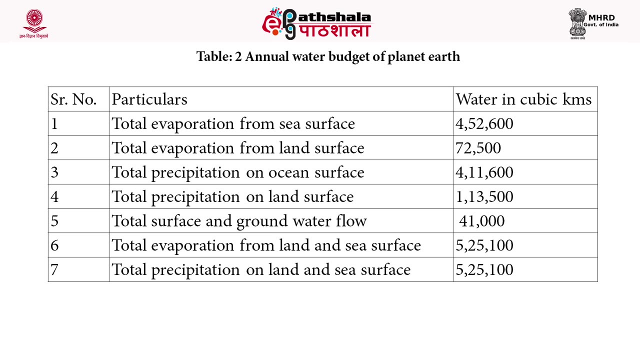 flow and affected by various climatic factors. Table 2 depicts the annual water budget of planet earth. From the table 2, it can be concluded that total evaporation from sea surface is 452500 cubic kilometer and total precipitation on land and sea surface is 525100. 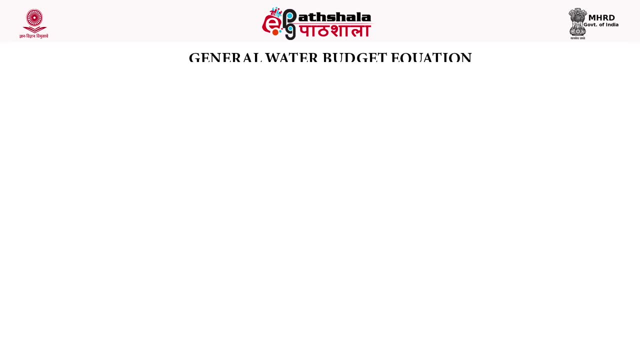 cubic kilometer. Now general equation to calculate the total, the water budget. it is P minus R, minus G, minus E minus T, equal to delta S, where P stand for precipitation, R stand for surface runoff, G stand for net ground water flow out of catchment. 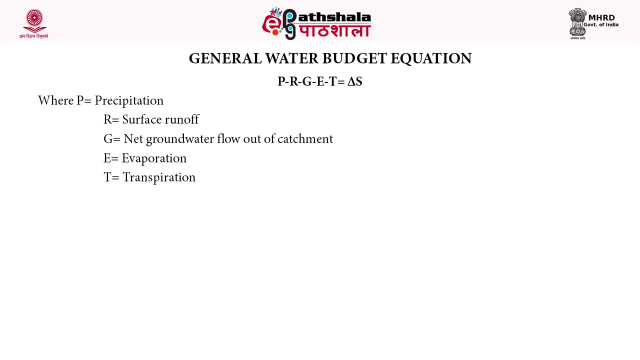 E stand for evaporation, T stand for transpiration and delta S is change in storage. All the terms equation have the dimension of volume, or we can also calculate water budget as water and any given location and time can be accounted as precipitation equal to evapotranspiration. 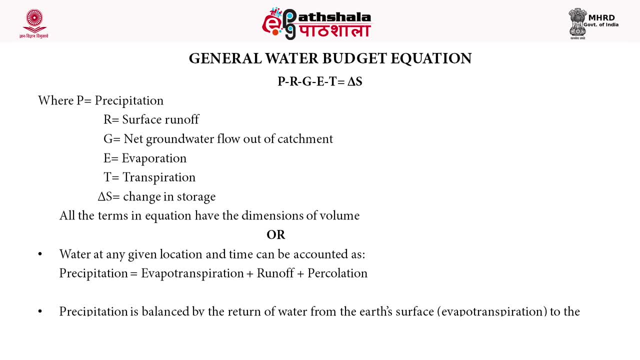 plus runoff per plus percolation, that is, water evaporated from earth surface reached by plants by the process of transpiration, runoff into ocean, river and percolate into ground water. If we have all these figure we can calculate the water budget of any particular area. Precipitation: 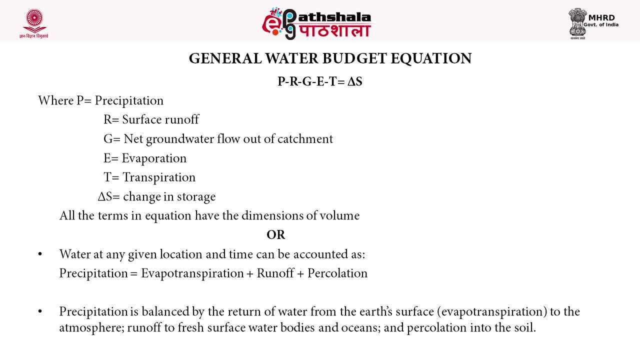 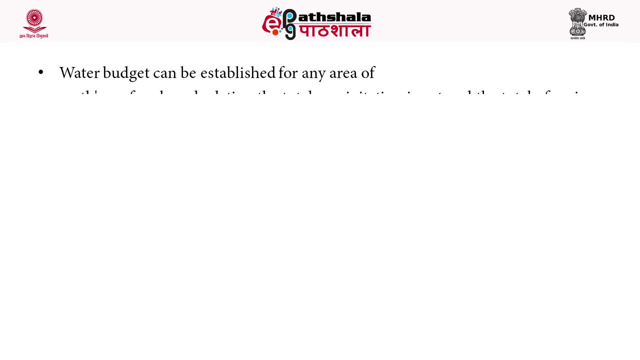 is balanced by the return of water from earth surface, that is, evapotranspiration, to the atmosphere, runoff to press surface water body and ocean and percolation into the soil. Water budget can be established by established for any area of earth surface, by calculating the total. 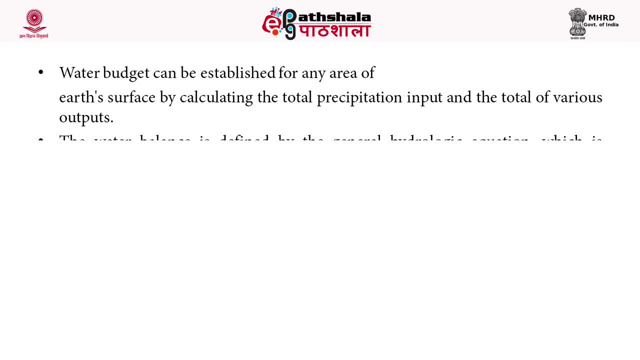 precipitation, input and total of various output. Input mean, that is rainfall. output mean used in various form, that is, in evaporation, transpiration, surface runoff, percolation, etcetera. The water balance is defined by the general hydrologic equation, which is basically a statement of: 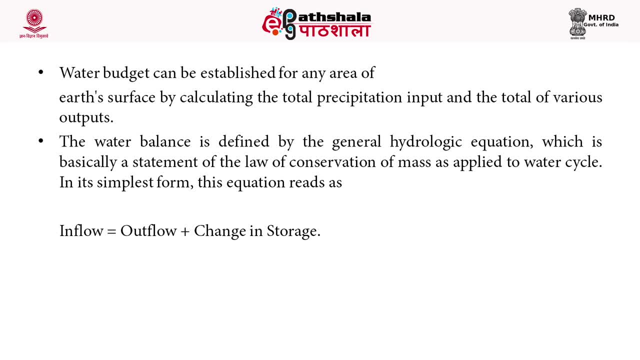 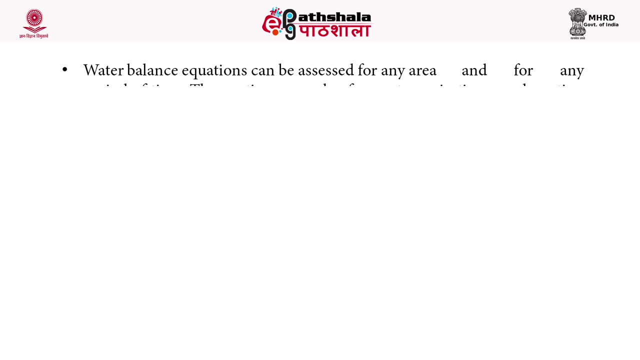 law of conservation of mass as applied to water cycle. In its simplest form, this equation reads as: inflow equal to outflow plus change in storage. Water balance equation can be assessed for any area and for any period of time. The continuous cycle of evapotranspiration. 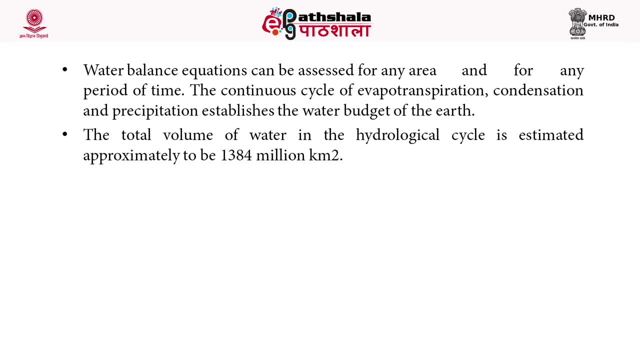 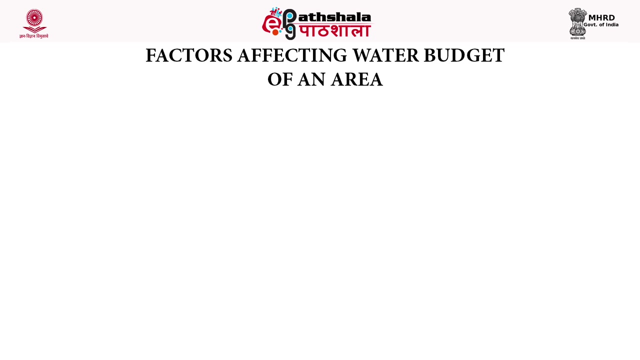 and precipitation establish the water budget of the earth. The total volume of water in the hydrological cycle is estimated approximately to be 1384 million kilometers square. Now we will discuss factors which affect the water budget of an area. These are wind seasons. 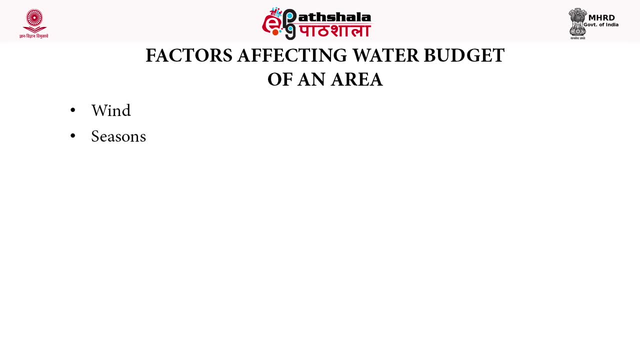 conditions, vegetation, temperature, precipitation, geographical location, that is, desert, etcetera, which have very less rainfall, Wind which move, collide from one place to another place, affect the rainfall Season. for example, in India, in monsoon we have maximum rainfall. 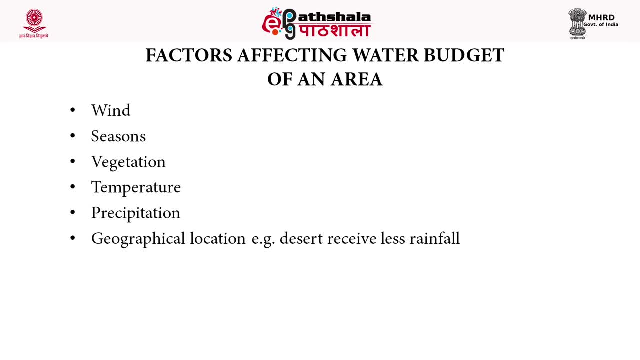 Vegetation. if we have more vegetation, more forest, it will release more water through the process. So we have more rainfall Temperature. we have more temperature, more evaporation, and all these factors ultimately affect the precipitation of any area. Now we will discuss about water budget of India. As we know, India has 18 percent population. 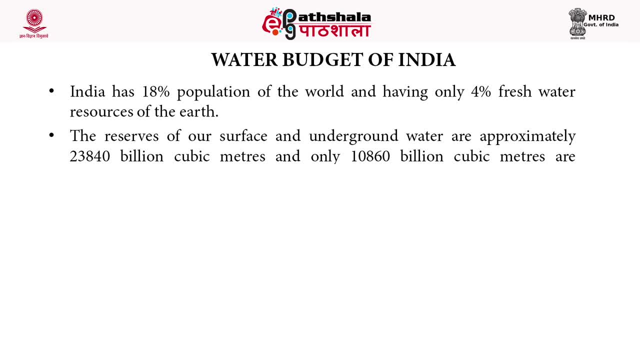 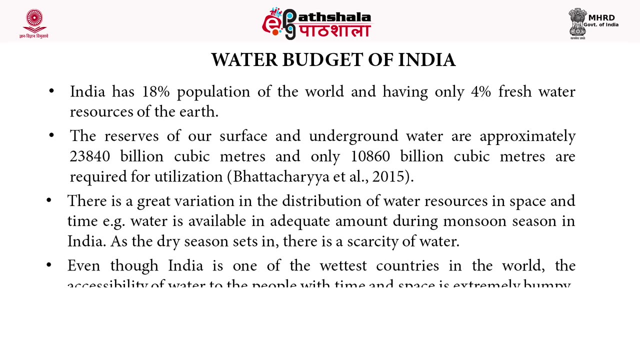 of the world and having only 4 percent fresh water resources of earth. The reserve of our surface and underground water are approximately 23,840 billion cubic meters, and only 10,860 billion cubic meters are required for utilization. There is a great variation in the distribution of water resources in space and time For 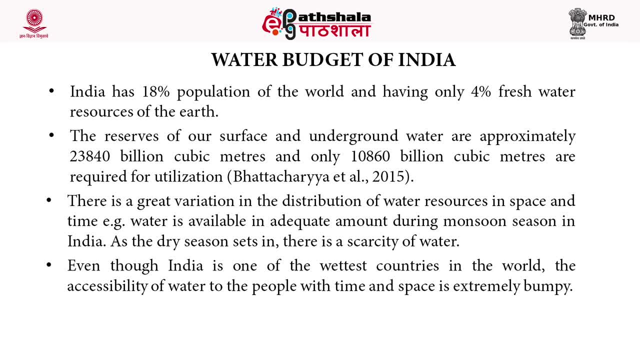 example, water is available in adequate amount during monsoon season in India. As the dry season sets in, there is a scarcity of water. For example, in India there is a large amount of water available in the monsoon season. As the dry season sets in, there is a scarcity. 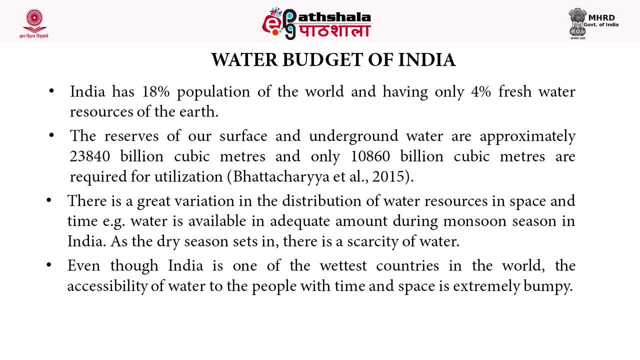 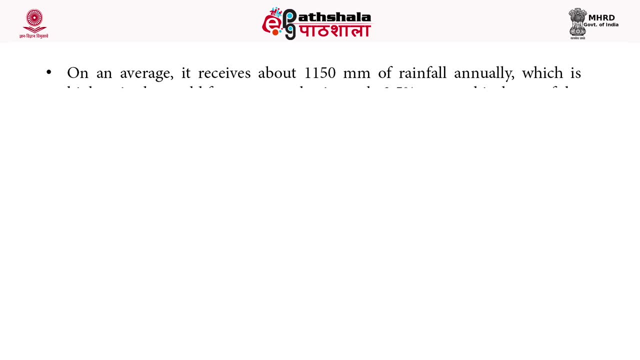 of water. There is a scarcity of water. Even though India is one of the wettest countries in the world, the accessibility of water to the people with time and space is extremely bumpy. On an average, it receives about 1150 mm, that is, millimeter of rainfall annually. 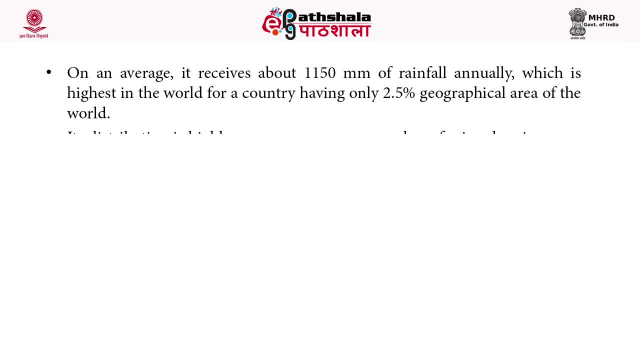 which is highest in the world for a country having only 2.5 percent geographical area of water. geographical area of the world. Its distribution is highly uneven. For example, average number of rainy days in year in India is only 40. Consequently, there is a lengthy curse of 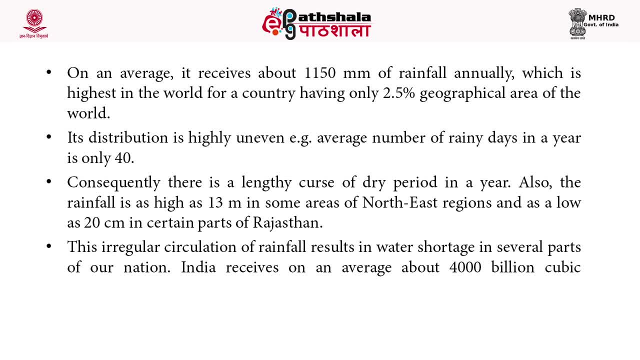 dry period in a year. Also, the rainfall is as high as 30 meter, 13 meter in some areas of north-east region and as low as 20 cm in certain parts of Rajasthan. The irregular circulation of rainfall results in water shortage in several parts of our country. India receive. 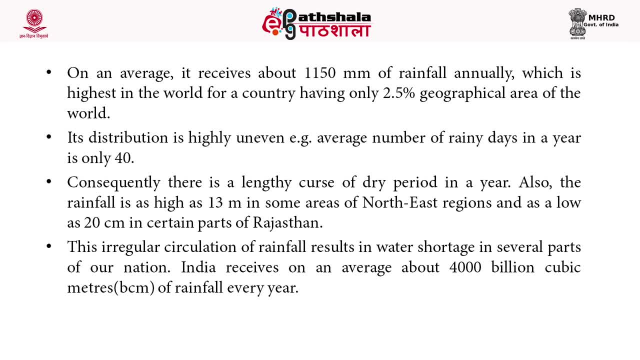 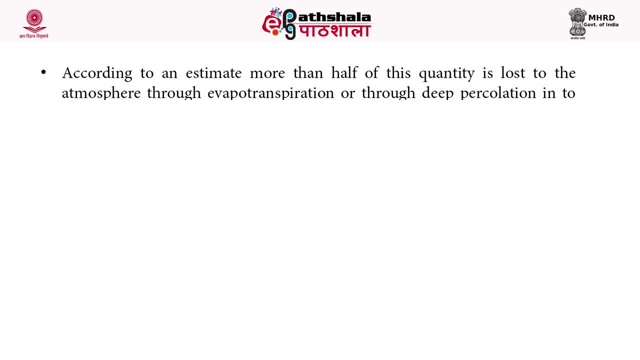 on an average, about 4000 billion cubic meters of rainfall every year. According to an estimate, more than half of this quantity is lost to the atmosphere through evapotranspiration or through deep percolation into groundwater, and only about 1869 billion cubic meter flow. 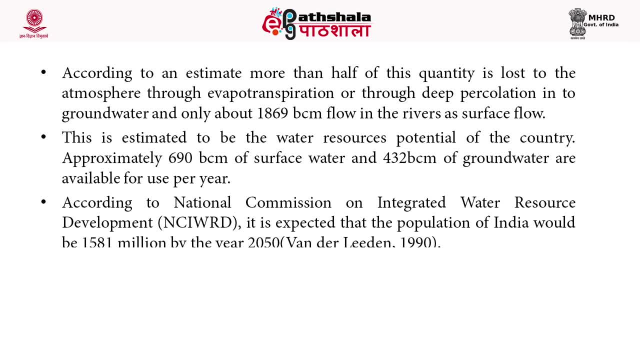 in the rivers as surface flow. This is estimated to be the water sources potential of the our country. Approximately 690 billion cubic meter of surface water and 432 billion cubic meter of groundwater are available for use per year, According to National Commission on Integrated Water Source Development. it is expected that 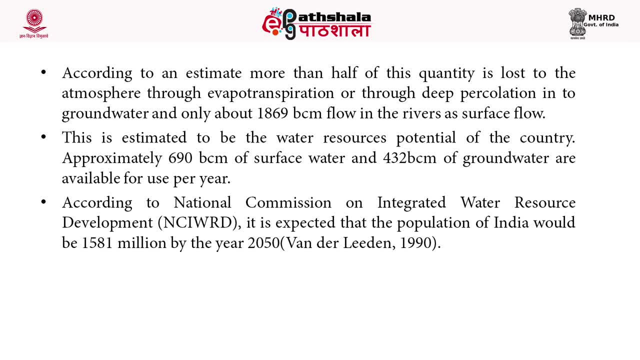 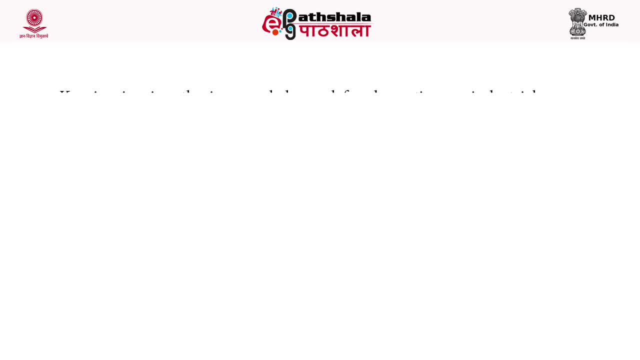 the population of India would be 1581 million by the year 2050.. That is more pressure on water sources. Keeping in view the increased demand for domestic use, industrial purpose, energy production, etc. and above all for agricultural production, there will be more demand of fresh. 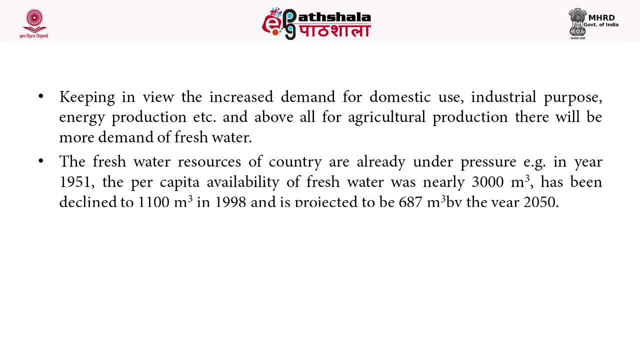 water. The fresh water resources of country are already under pressure. For example, in year 1951, the per capita availability of fresh water was nearly 3000 m3, 3000 m3 has been declined to 1100 m3 in 1998 and it projected to be 687 m3 by the year 2050.. The central water. 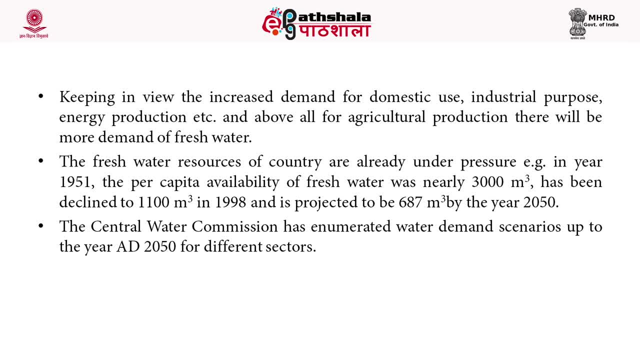 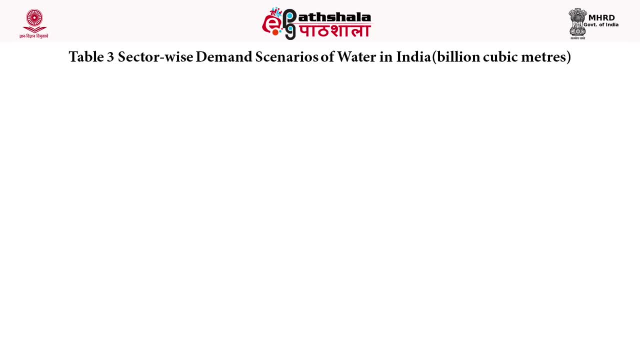 commission has enumerated water demand scenario up to the year of AD 2050 for different sector and it is shown in table 3.. For example, for irrigation, we need 910 billion cubic water for irrigation only in 2025 and the figure will increase up to 1072 billion cubic meter in 80th century. 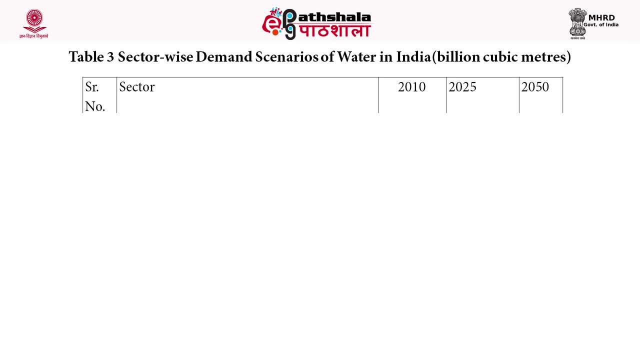 We need double thearden- Idaho Nile present and the Roda river Loop present and the Central Water Korner Project Demo, and we had a data, which was published about this in our table 2013, that the właśnie hydro printer HDG, which manages the general water level from west to south, can produceamar delete water. collects elements from west to west. Due to these adel manus, nine billion cubic met gram per meter amount has been increased on a daily basis here after this. In the past the great rule was that in the summer union we had to, and now we have to, extend this value of the total allocation of solar power registers. 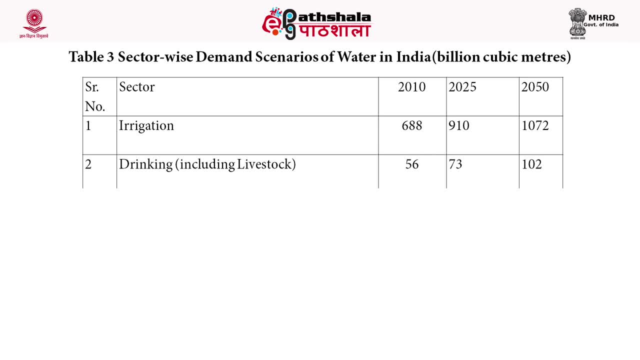 water for irrigation only in 2025, and the figure will increase up to 1072 billion cubic meter in year 2050.. Likewise, irrigation: drinking: in drinking, we need 73 billion cubic meter water in 2025,, and it will be increased to 102 billion cubic meter in 2050.. Likewise, 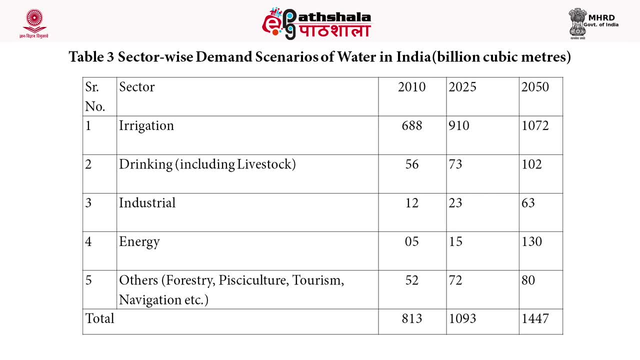 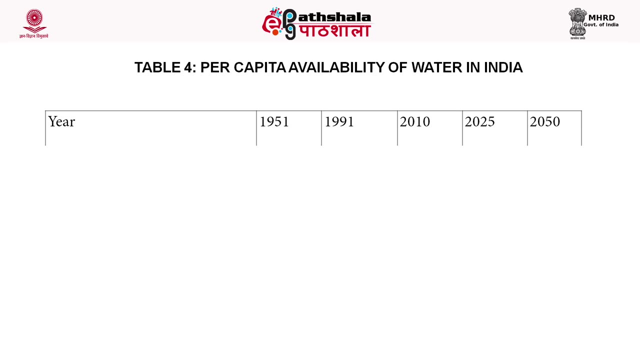 these. in various sectors, that is, industry, energy demand and other, that is forestry, physical, tourism, navigation, etcetera- the demand for fresh water will be increased definitely. The table 4 shows per capita availability of water in India, For example in 1951, it. 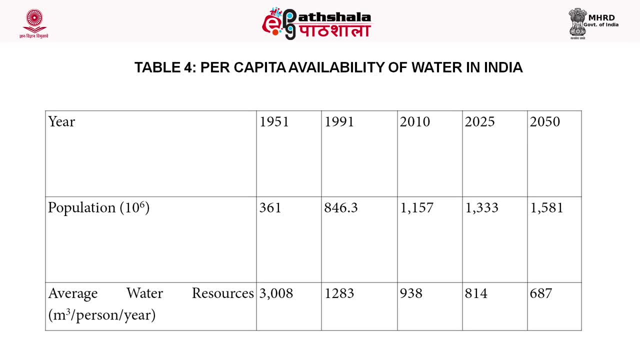 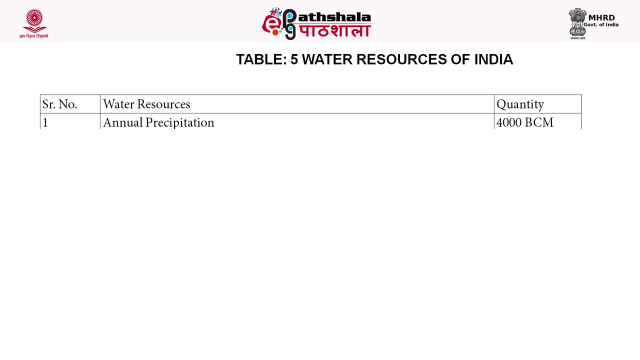 was 360 billion cubic meter 360, and in 2050, it will be 3.5 billion cubic meter, and in 2050, it will be 3.5 billion cubic meter. Moreover, table 5, enumerate the water sources of India. For example, in India we have annual 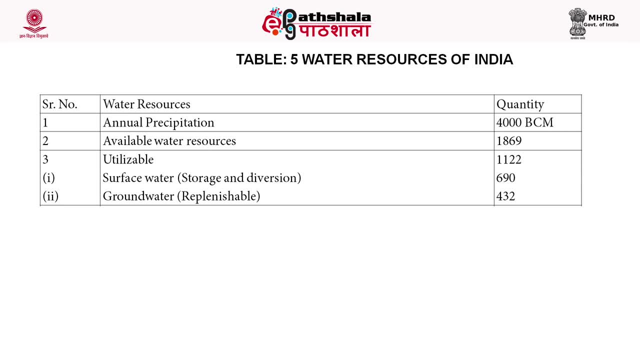 precipitation, that is, rainfall, is 4000 billion cubic meter. From these available water sources, 1869 million cubic meter. We are utilizing surface water and ground water. that is, 690 billion cubic meter and 432 billion cubic meter. Presently, we are using 605 billion cubic meter of fresh water. 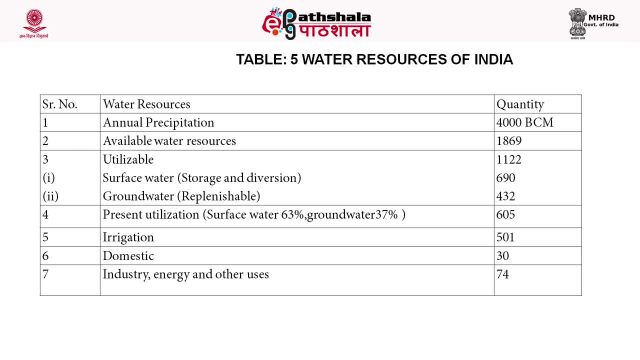 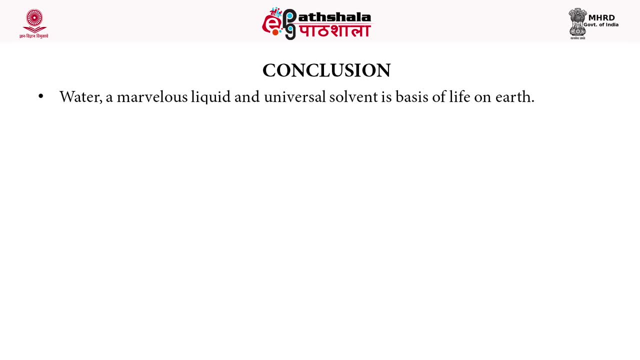 that is, from surface and ground water collectively. Conclusion: Water, a marvellous source of water, is a water source of fresh water. It is a biodegradable, natural and natural water. It is a natural water source. It is a liquid water source. It is a natural water source. Its base is a. 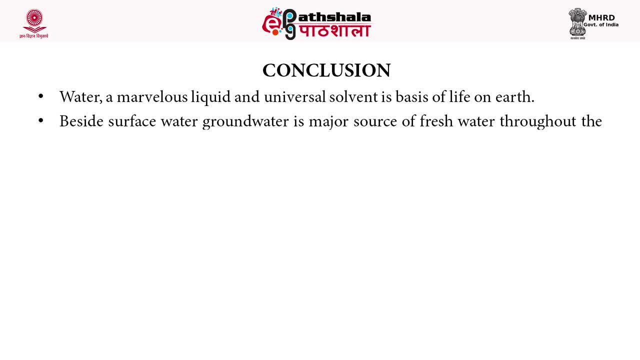 light liquid and a universal solvent. Its base is a life on earth. Besides surface water, ground water is a major source of fresh water throughout the world. Due to human activity, surface and ground water quality is deteriorating day by day. Besides these anthropogenic activities,